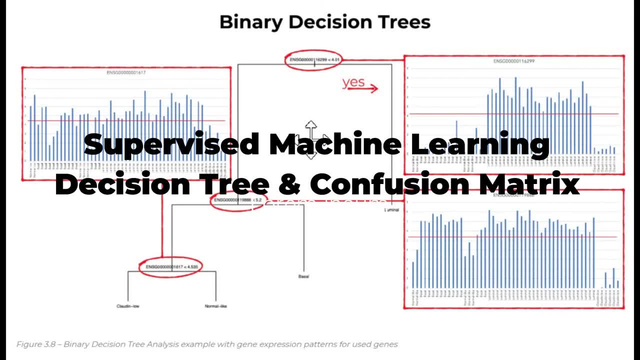 Hello, today we are going to talk about decision trees and random forest. Decision tree is a type of a classification algorithm. Each decision tree is created by rules. Binary means the branch, that can be either yes or no, and if the expression of a gene is. 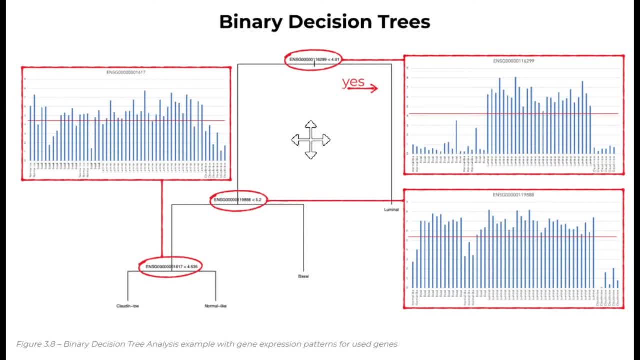 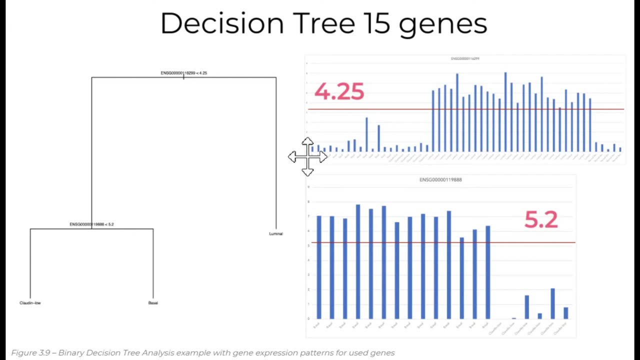 higher than x, the classes will separate. For example, in the figure here you can see that the lumenant class can be separated from all the other classes based on the gene ANSG00000016299.. This rest of the samples are further divided into the other classes based on other genes that are: 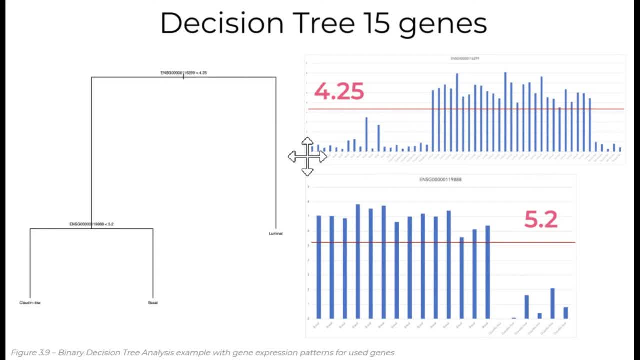 separating this group into cloud and low, normal, like and basic classes. The algorithm will continue to run until it has effectively separated all the samples into some group. If we use less than or equal to the number of classes, then the number of classes will be less than or equal to. 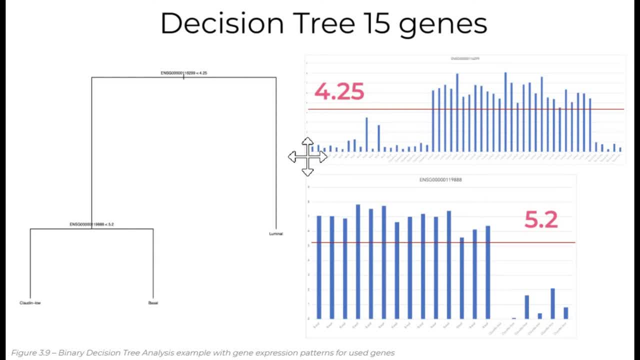 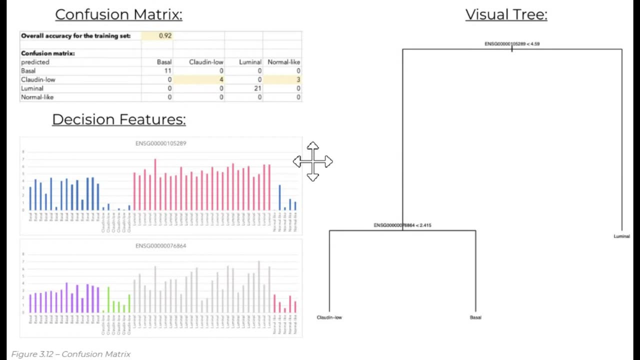 the number of classes. In this second example of a binary decision tree for breast cancer gene expression table we see the data is separated into three groups: luminal, basal and cloud and low, with only two genes. Binary decision trees are initiated in a random start, so the genes 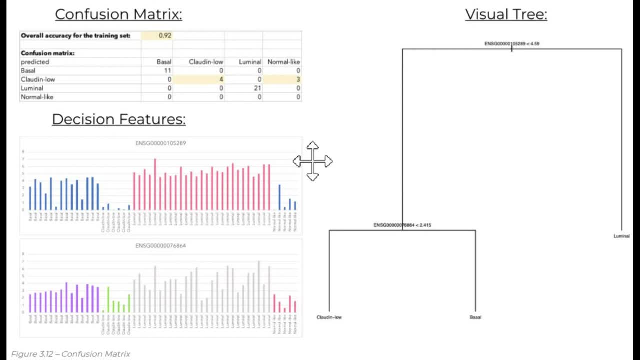 selected in the procedure can change from time to time. To try running decision tree pipeline on the server, select the supervised learning section and area of analysis where you are going to upload the training and the test data, and select the decision trees button in the pipeline builder. So let's get started. Upload your data. 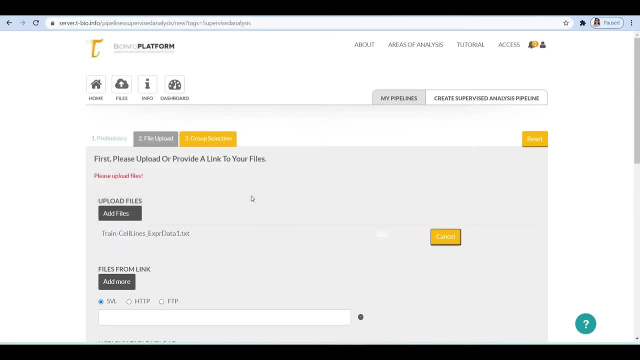 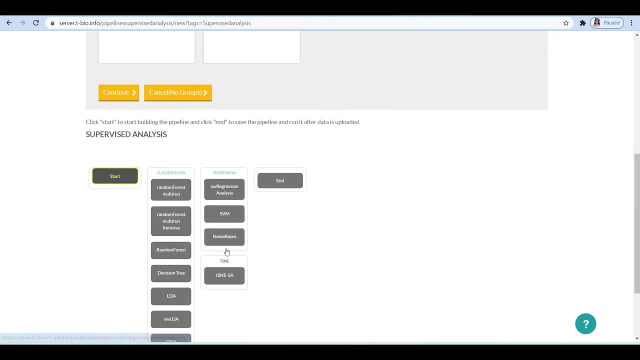 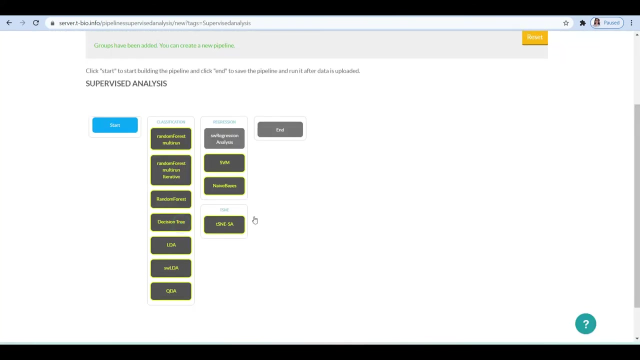 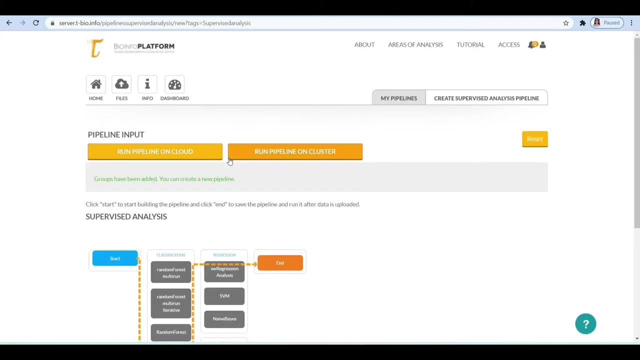 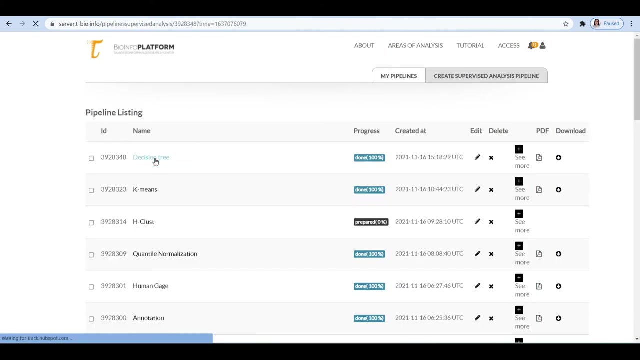 and now, once the upload is finished, select your train and test data. Now click on start and click on decision tree. Now end your pipeline, give a name to your pipeline and stay updated with the status of your pipeline timely by checking the pipelines In the results. 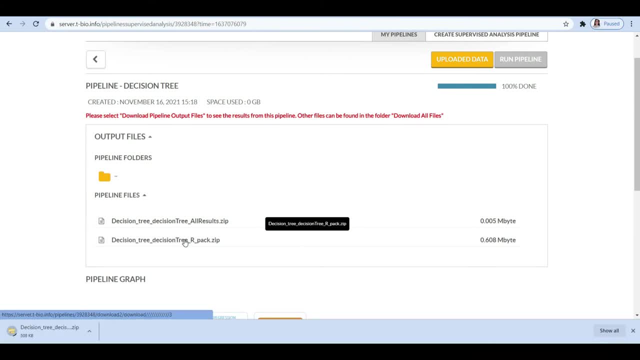 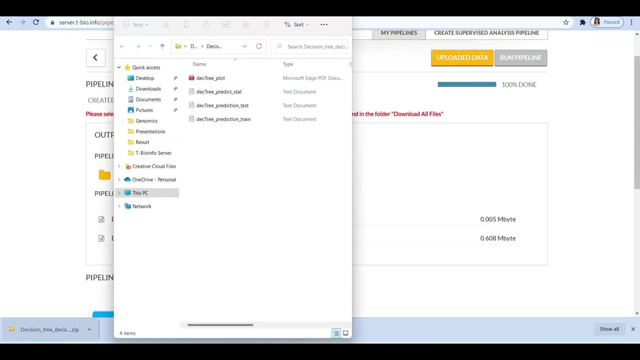 you will see the prediction for test set and the PDF with the decision tree visualization For your. Also, you would obtain a confusion matrix that reveals an issue that the algorithm ran into. Cloud and low was identified 4 times as cloud and low and 3 times as normal. like